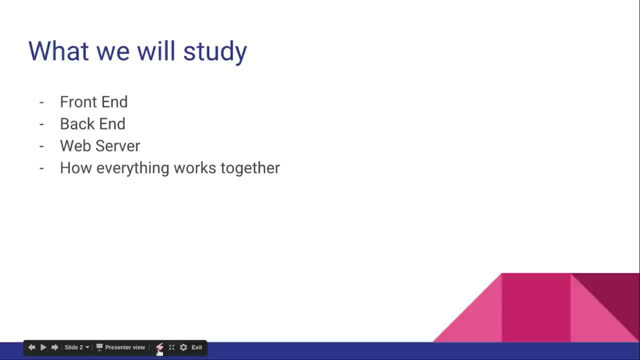 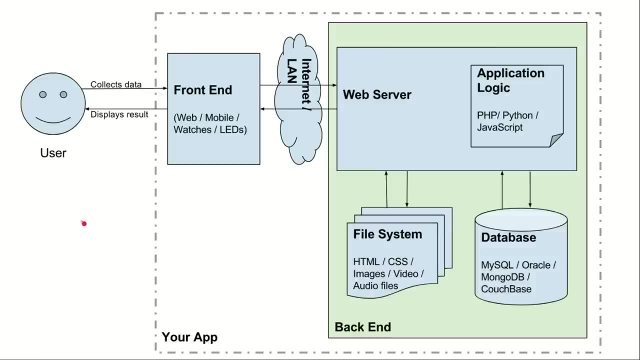 let's start with our video. okay, so we have got this ginormous diagram, but don't worry, i'm going to explain each and every single thing out that is there in this diagram. okay, so it all starts with a user. a user has learned about this new application which has been introduced and all of 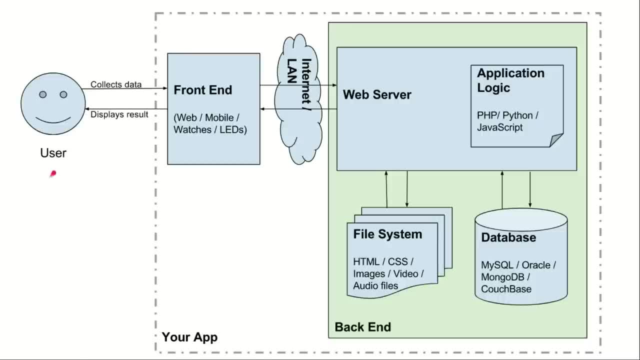 the people are going crazy over this application, so user thinks that it will be a good idea to try this application out. so he wants to try your application right now. your application can be a web application which runs on ios or android devices. or it can be a web application or it can. 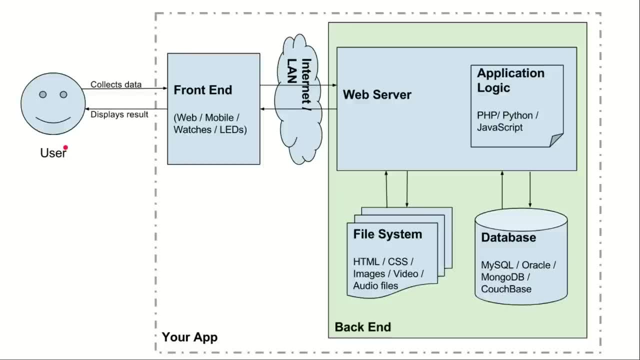 be a desktop application as well. so user downloads your application or goes to your website and what he sees in the very beginning is known as the front end. now the responsibility of the front end is to collect the data from the user and hand the data the backend so that backend can act upon that data, process that data, store that data for. 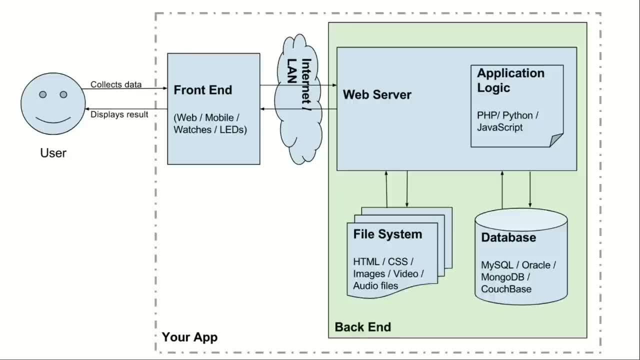 future retrievers and return the processed output to the user. That is how user gets something out of your application, right? So frontend can contain forms. frontend can contain other UI element which enables the user to create the data on your application and that data is passed from the frontend. 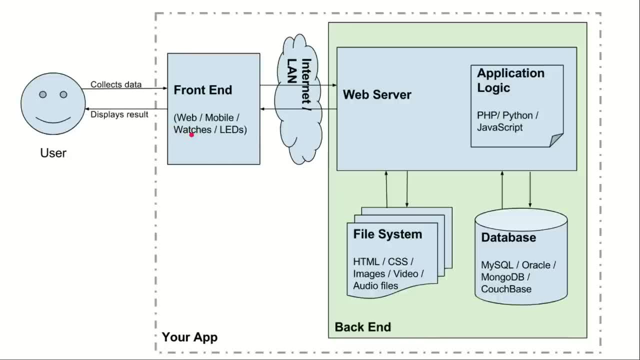 to the backend right. So your frontend can be anything. It is just a user interface which enables user to do something. So it can be a website or a web application or a single page web application. It can be your Android or iOS mobile application. 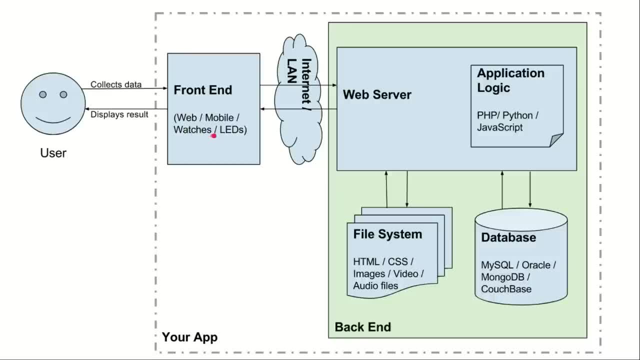 It can be the new smart watches application or it can be something like LEDs and buttons and things like that. So your TV remote is also a frontend. It has some buttons over it which you can press and once you press a button, a data is generated and that data is passed on to the backend of your TV or whatever your remote. 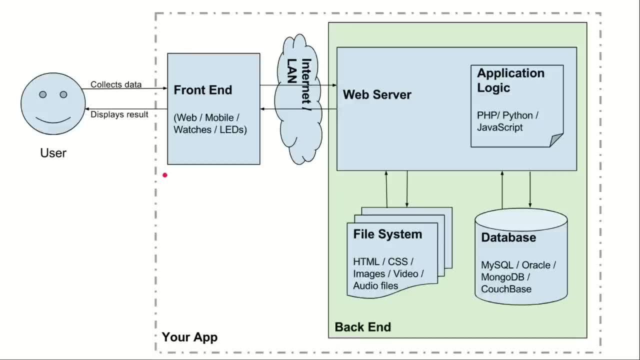 is controlling. So that is all about frontend And it is all about collecting the data from the user and displaying the result to the user. Okay, So how the data which is collected from the user is transferred to the backend. Most of the time, internet is involved in transferring the data. 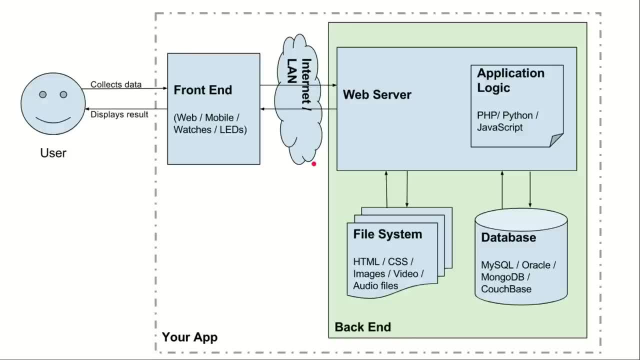 The most common way of transferring the data from the frontend to the backend is using the internet. So internet can be the web or it can be local networks, But the protocol which is being used to transfer the data most of the time is HTTP protocol. 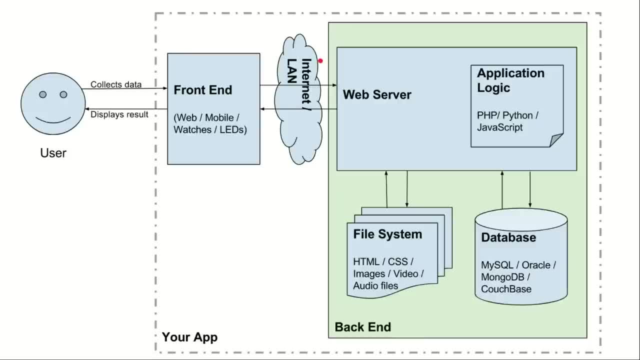 Now, if you are not clear about how internet works and how data gets transferred from one computer to another computer which is sitting across the globe, maybe you should go out and check my other video where I have explained internet. So internet can be the web or it can be local networks. 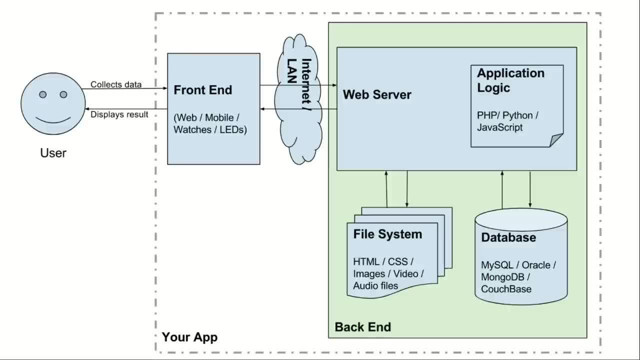 I have explained everything about how internet works, right. So the data is transferred from the frontend to the backend using the HTTP protocol. Now, once this data is transferred to the server, there is an agent, or you can call it a gatekeeper, which is known as the web server. 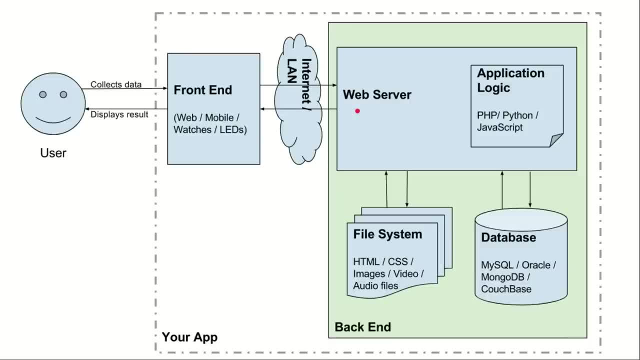 Now, once web server gets the data, it can act upon it right. So web server, Most of the time, Most of the time- comes with a lot of plugins, and these plugins actually help you to run the code in various languages. like you can run PHP, you can run JavaScript applications. 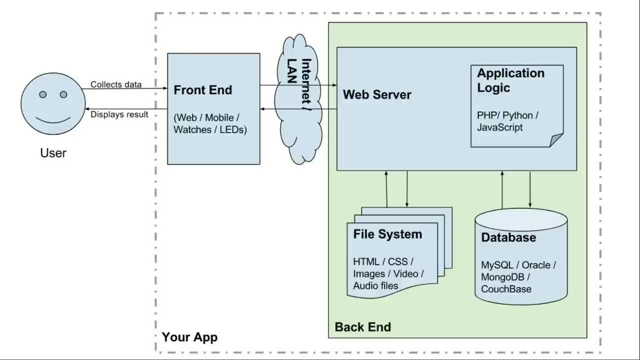 you can run ASPNET as well and there are several other programming language support which is available for web servers. Now web server has a primary responsibility of serving the files over the internet to the user Because this user requests for abcpng right. So frontend will collect the file name which user wants to retrieve. okay, 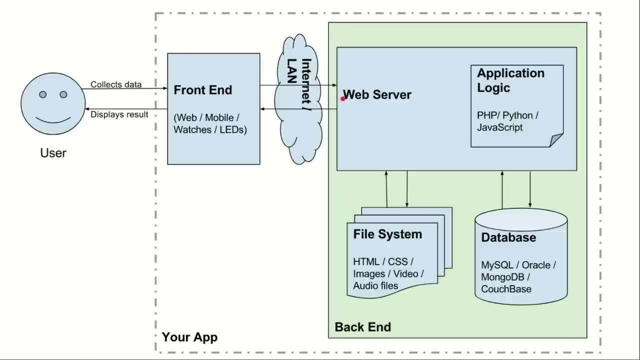 So abcpng file name is passed on to this web server. Now web server can straight head over to the file system of your operating system, okay, And it can search for abcpng in the file system And it can directly return that file name. 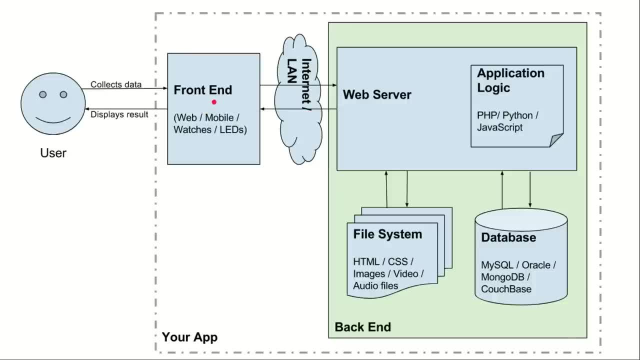 Okay, And it can directly return that file to the user and this frontend can display that file. So in that case web server does not have to deal with any dynamic content. It just go out, search for the HTML or CSS or whatever file and it directly returns that. 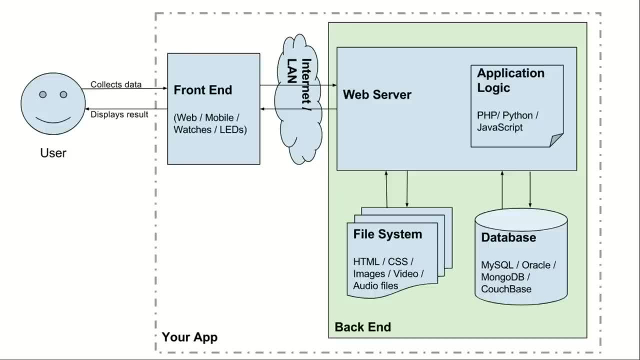 file to the user. So that is a primary responsibility of a web server. It serves the request it receives from the frontend- okay, And that frontend is getting the request eventually from the user. Okay Now web servers also come with various functionalities, like you can plug in your application logic. 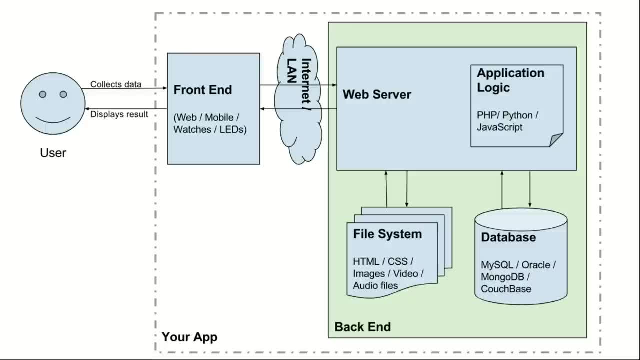 so that the application logic can perform several other checks or whatever the business logic requires on to that received data. And just in case it wants to store that particular data, it can interact with the database layer using server. So it can use several mechanisms like ORM and connectors and store the data for the 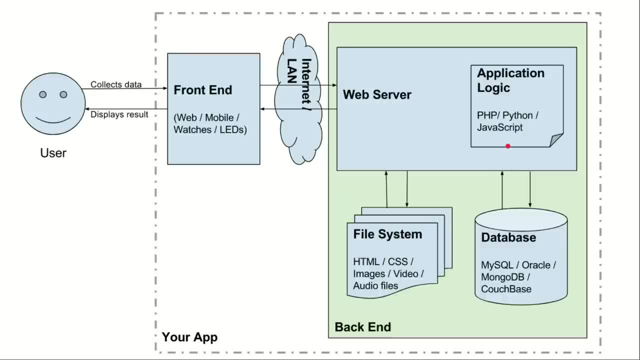 future retrievals right And once that application logic has performed its cleanup activities or whatever the business logic requires, it returns the data over to the web server. right Now web server has got its data. Now it can return the data to the frontend. 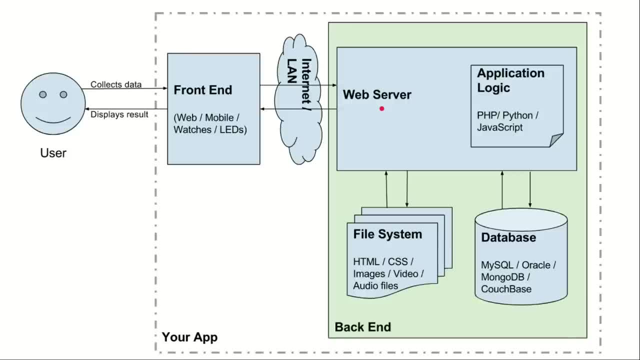 So in that particular sense, web server can actually do that, Okay, Okay, So web server can actually help in serving dynamic web pages or dynamic application. So in this particular case, web server was directly serving you the files it already knows about. 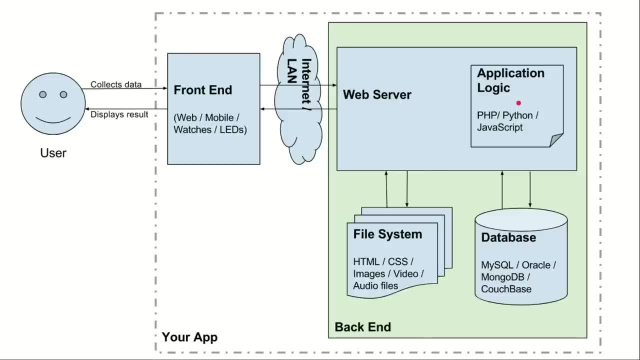 But in case the application logic generates the file and that file is generated on the fly using the data and performing some operations on the data, and that dynamic file is returned to the web server using server. So this is the application logic layer. All of this stuff was happening in the background and this whole layer of web server file system. 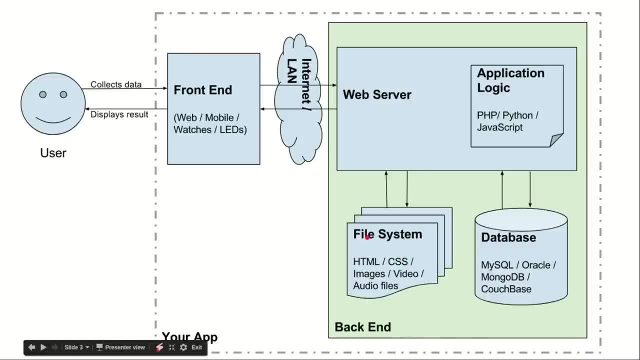 and database is far removed from the user and it can be located anywhere across the globe. It is a responsibility of the frontend to pass the data over to the right server. right, And all of these components together, Okay, Okay, Okay. All of these components together are known as the backend of your application. 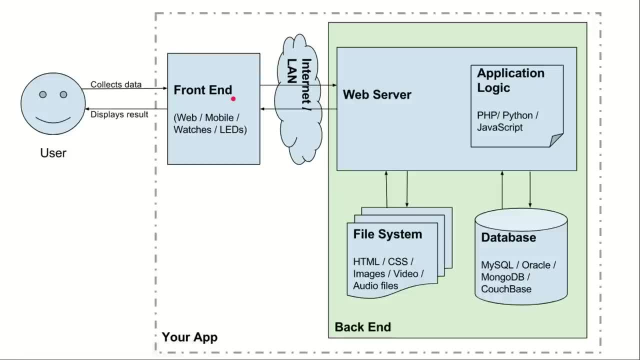 So now you have the working understanding of what comprises of a frontend and what makes a backend right, And when we put all of these together, you get your app. So now, if you are going to launch an Android app, that Android app, which resides on user's 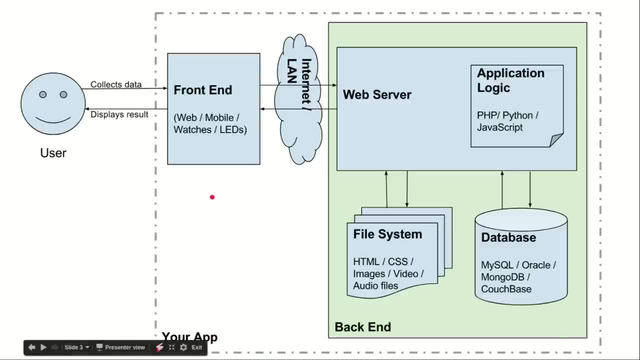 mobile will comprise of a frontend. Okay, can eventually also perform some kind of business logic, but that business logic will only be persisting if you pass that data to your backend, right? so if you want to persist any kind of data, you need some kind of backend, and most of the time the backend resides on some servers which are far 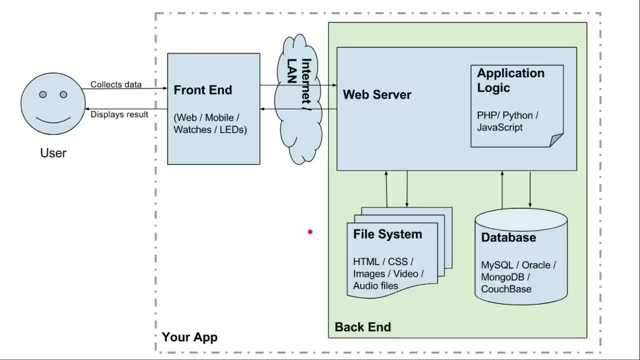 removed from the user. so you will establish some kind of server for your application which will store the data of all of your users for future retrieval and performing some critical business operations, right? so i hope that now you are very clear about how everything works and what kind of 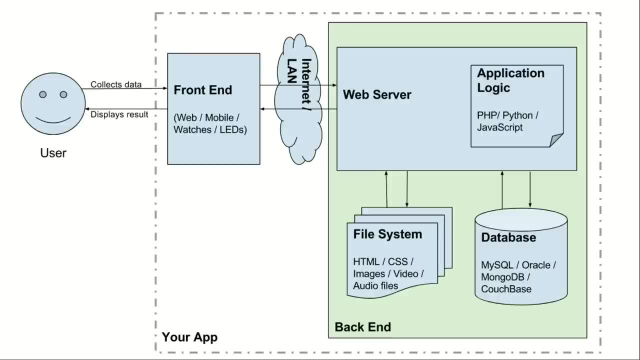 component you will actually require in order to create a working modern day application. so that's it for today's video. thank you for watching and i will see you in the next video. this is just a basic overview of how everything is laid out and how everything works in my next. 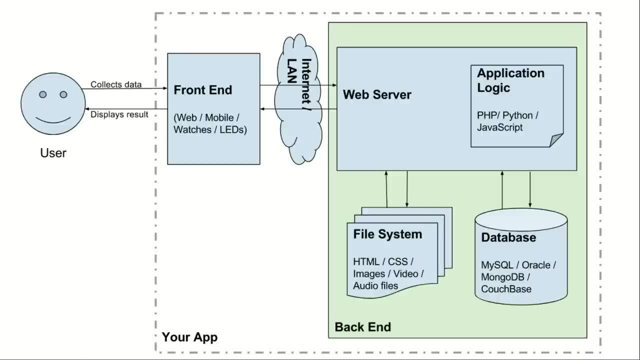 video. we are going to talk about several other nitty-gritty things which can be put into this ecosystem so that your application can be fast enough. we are going to talk about load balancers, catching and several other things, so make sure if you want to be educated about even better.